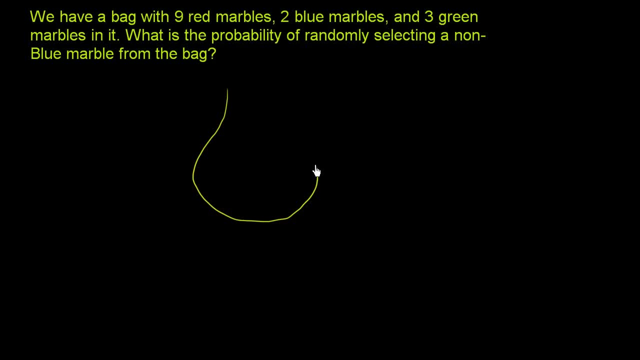 So let's draw this bag here. So that's my bag, And we're going to assume that it's a transparent bag That looks like a vase. But we have nine red marbles. So let me draw nine red marbles: One, two, three, four, five, six, seven, eight. 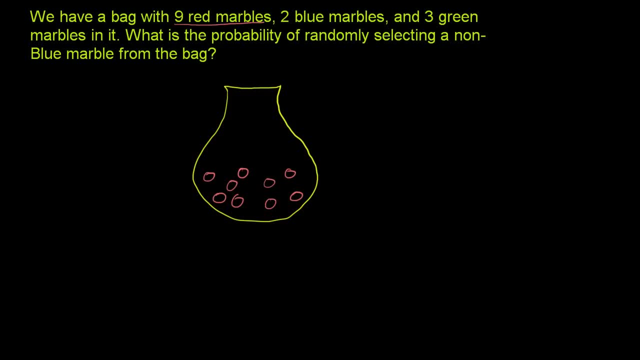 nine red marbles, So that looks kind of orangish but does the job. Two blue marbles. So we have one blue marble, two blue marbles, And then we have three green marbles. Let me draw those three. So one, two, three. 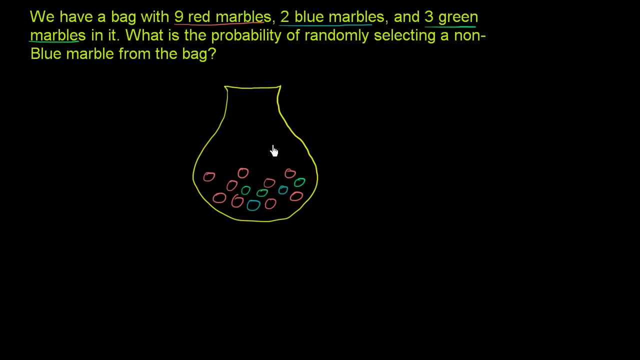 What is the probability of randomly selecting a non-blue marble from the bag? So maybe we mix them all up and we have an equal probability of selecting any one of these, And the way you just think about it is what fraction of all of the possible events? 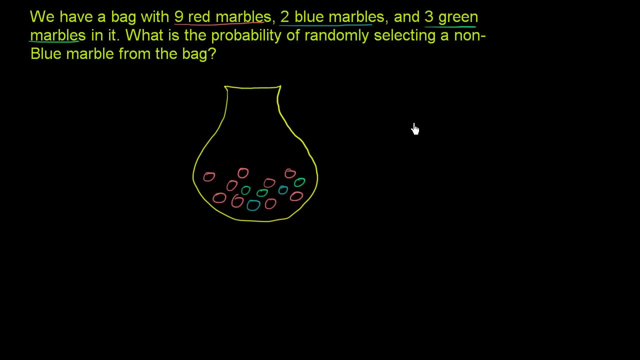 meet our constraints. So let's just think about all of the possible events first. How many different possible marbles can we take out? Well, that's just the total number of marbles there are. So there are 1, 2,, 3, 4, 5, 6, 7, 8, 9, 10,, 11,, 12,, 13, 14. 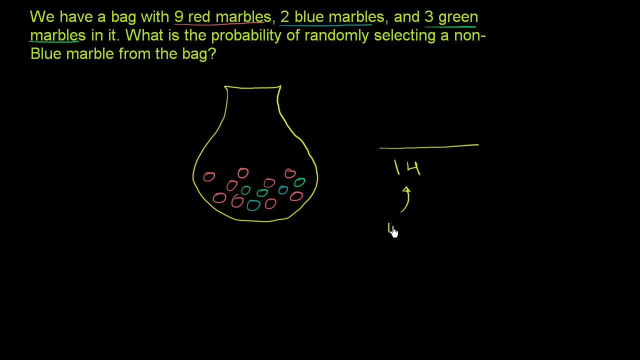 possible marbles. So this is the number of possibilities, And then we just have to think what fraction of those possibilities meet our constraints. And the other way you could have gotten 14 is just taking 9 plus 2 plus 3.. 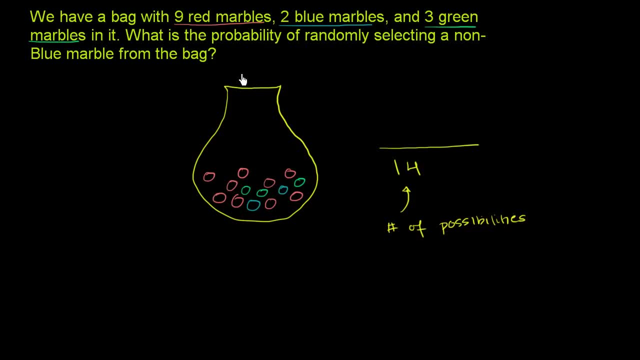 So what number of those possibilities meet our constraints, And remember our constraint- is selecting a non-blue marble from the bag. Another way to think about it is a red or a green marble, because the only non-blue ones, the other two colors we have- 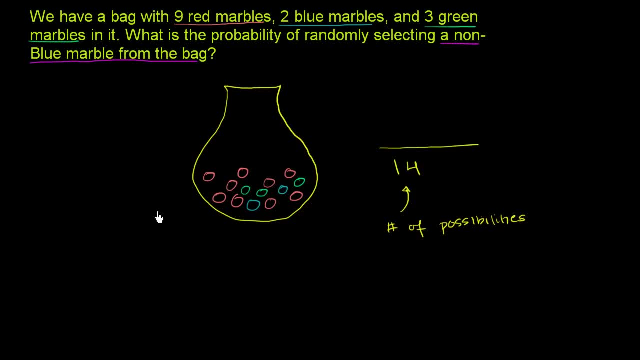 are red and green. So how many non-blue marbles are there? Well, there's a couple of ways to think about it. You could say there's 14 total marbles. Two are blue. so there are going to be 14 minus 2,. 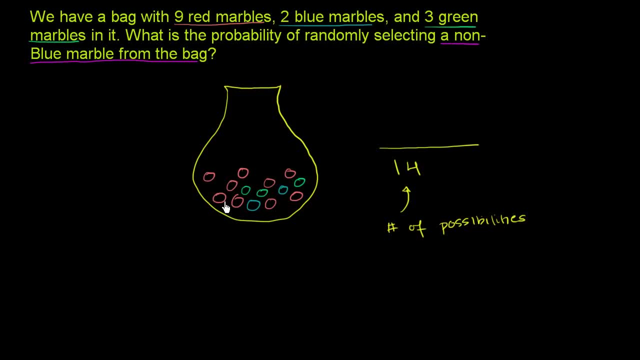 which is 12 non-blue marbles, Or you could just count them 1,, 2,, 3,, 4,, 5, 6, 7,, 8,, 9,, 10,, 11, 12.. 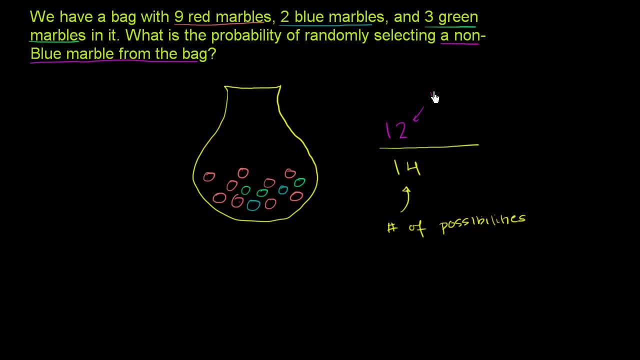 So there are 12 non-blue marbles. So that's the number of non-blue. So these are the possibilities that meet our constraints over all of the possibilities. And then, if we want to, this isn't in simplified form right here, since both 12 and 14 are divisible by 2.. 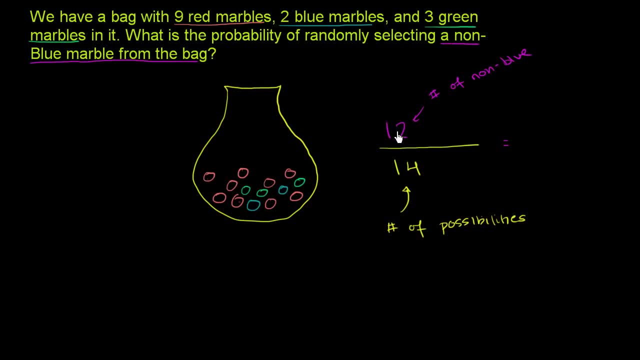 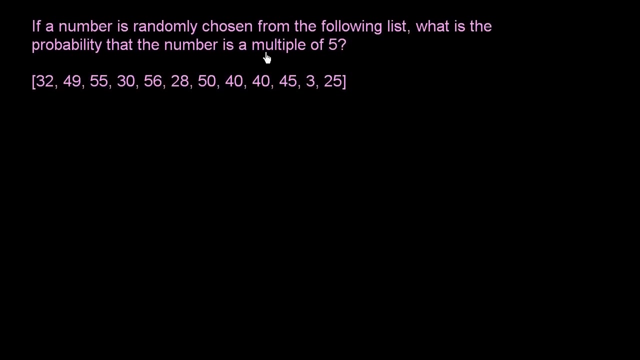 So let's divide both the numerator and the denominator by 2, and you get 6 over 7.. So we have a 6. seventh chance of selecting a non-blue marble from the bag. Let's do another one If a number is randomly chosen. 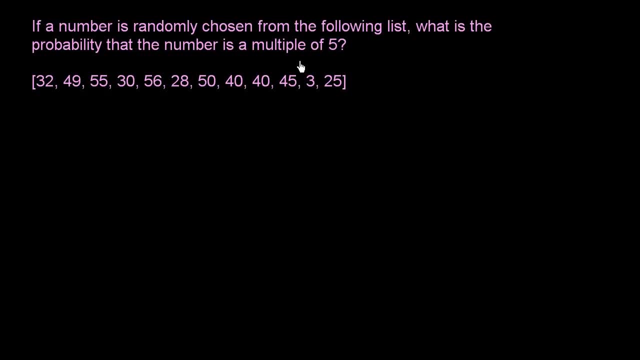 From the following list. what is the probability that the number is a multiple of 5?? So, once again, we want to find the fraction of the total possibilities that meet our constraint, And our constraint is being a multiple of 5.. So how many total possibilities are there? 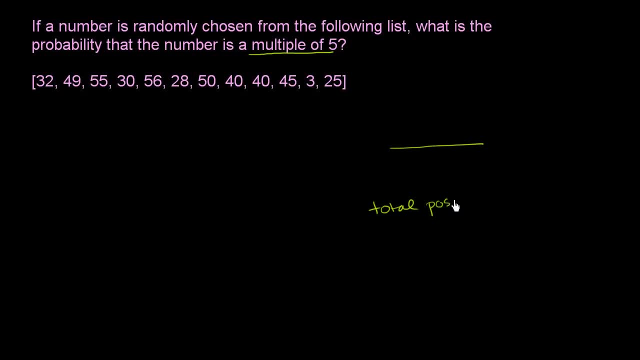 Let's think about that. Total possibilities, How many do we have? Well, that's just the total number of numbers we have to pick from. So 1, 2, 3.. 3, 4, 5, 6, 7, 8, 9, 10,, 11,, 12.. 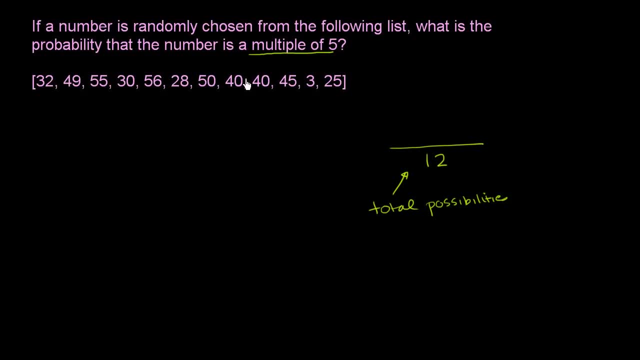 So there are 12 possibilities. We have an equal chance of picking any one of these 12.. Now, which of these 12 are a multiple of 5?? So let me do this in a different color. So let me pick out the multiples of 5.. 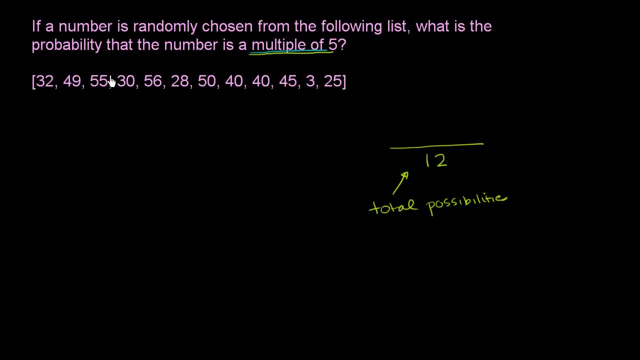 32 is not a multiple of 5.. 49 is not a multiple of 5.. 55 is a multiple of 5.. Really, we're just looking for the numbers that in the ones place either have a 5 or a 0.. 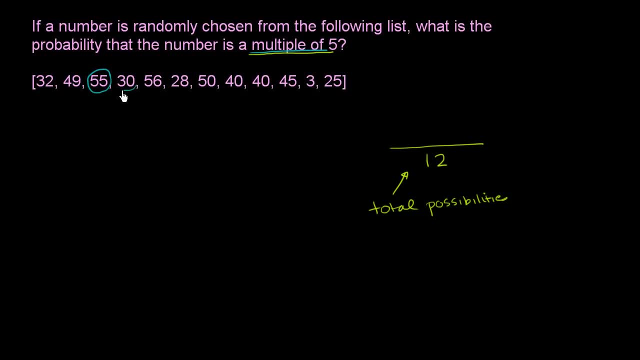 55 is a multiple of 5.. 30 is a multiple of 5.. That's 6 times 5.. That's 55 is 11 times 5.. Not 56, not 28.. This is clearly 5 times 10.. 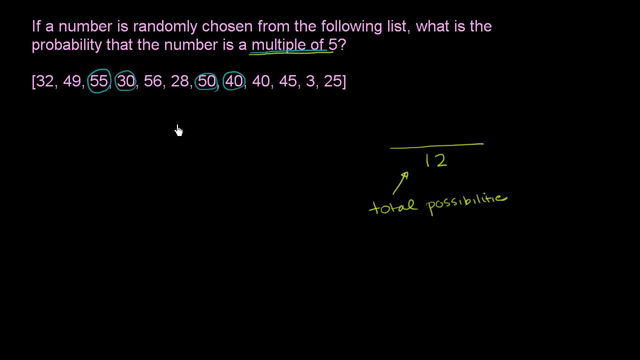 This is 8 times 5.. This is the same number, again Also 8 times 5.. So all of these are multiples of 5.. 45, that's a 9 times 5.. 3 is not a multiple of 5.. 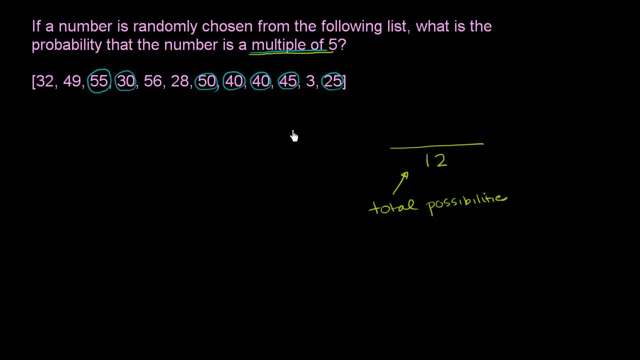 25, clearly 5 times 5.. So I've circled all of the multiples of 5.. So, of all the possibilities, there's possibilities, The ones that meet our constraint of being a multiple of 5, there are 1,, 2,, 3,, 4,, 5,, 6,, 7 possibilities. 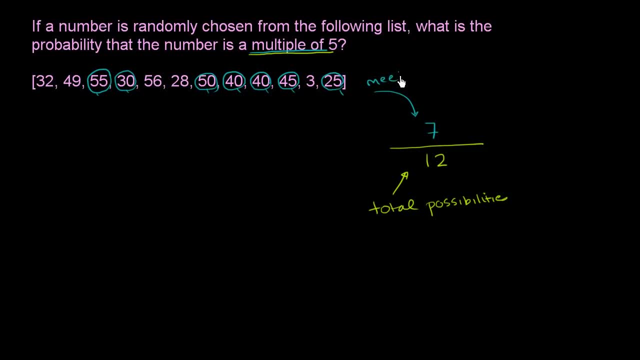 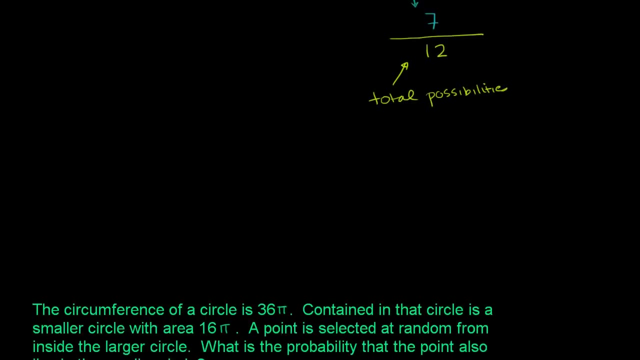 So 7 meet our constraint. So in this example, the probability of selecting a number that is a multiple of 5 is 7 twelfths. Let's do another one. The circumference of a circle is 36 pi. Let's draw this. 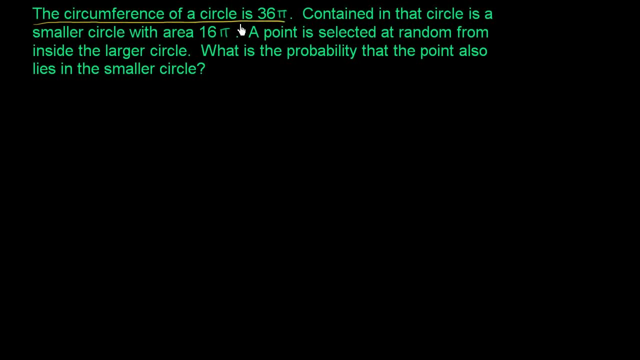 Let's draw this circle. The circumference of a circle is 36 pi. So let's say the circle looks. I can draw a neater circle than that. So let's say the circle looks something like that And the circumference. we have to be careful here. 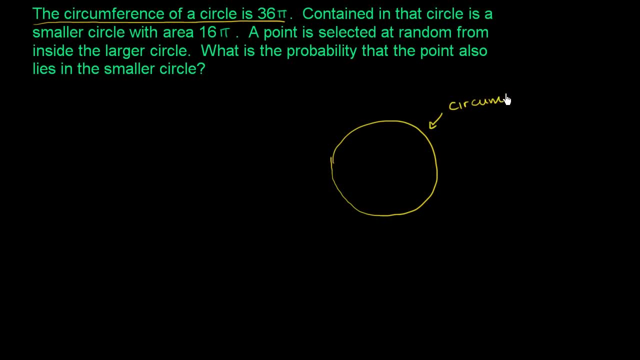 They're giving us interesting. so circumference, The circumference is 36 pi. Then they tell us that contained in that circle is a smaller circle with area 16 pi. So inside the bigger circle we have a smaller circle that has this guy right over here has an area of 16 pi. 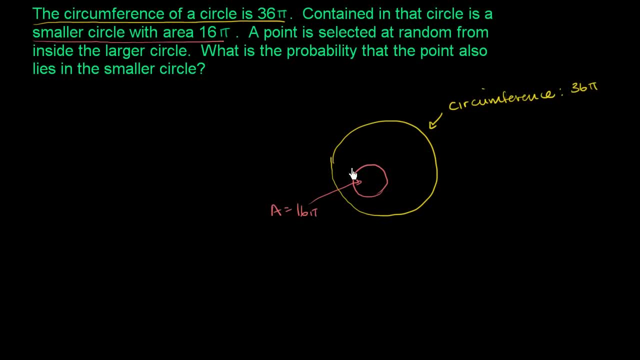 A point is selected at random from inside the larger circle. So we're going to randomly select some point in this larger circle. What is the probability that the point also lies in this smaller circle? So here it's a little bit interesting, because you actually have an infinite number of points. 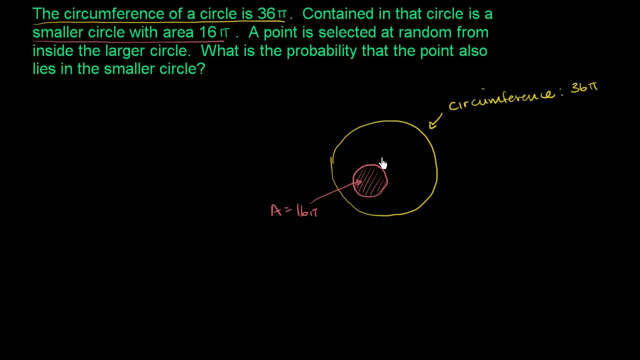 in both of these circles, Because it's They're not. it's not. it's not kind of separate balls or marbles, like we saw in the first example, or separate numbers. There's actually an infinite number of points you can pick here. 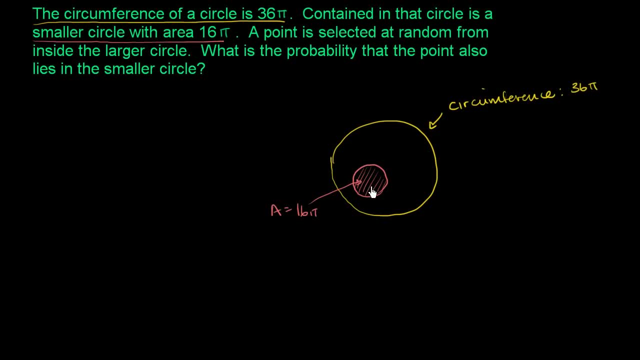 And so when we talk about the probability that the point also lies in the smaller circle, we're really thinking about the percentage of the points in the larger circle that are also in the smaller circle, Or another way to think about it is the probability. 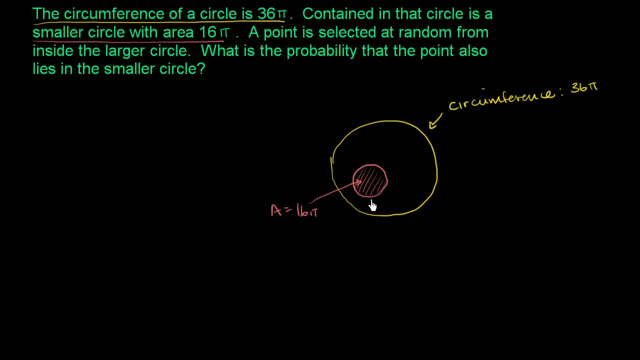 that the point is also the probability that if we were to pick a point from this larger circle, the probability that it's also in the smaller circle is really just going to be the percentage of the larger circle that is the smaller circle. I know that might sound confusing. 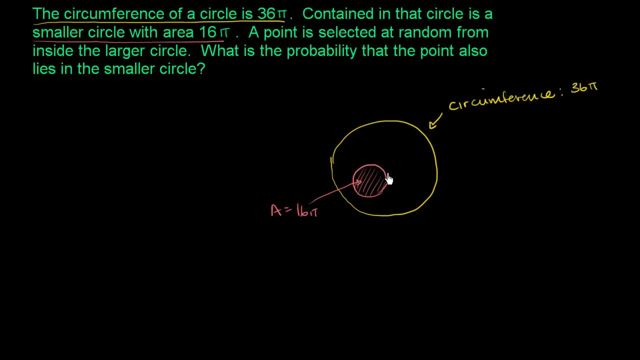 But we really just have to figure out the areas for both of them And it's really just going to be the ratio. So let's think about that. So there's a temptation to just use this 36 pi up here, But we have to remember this was the circumference. 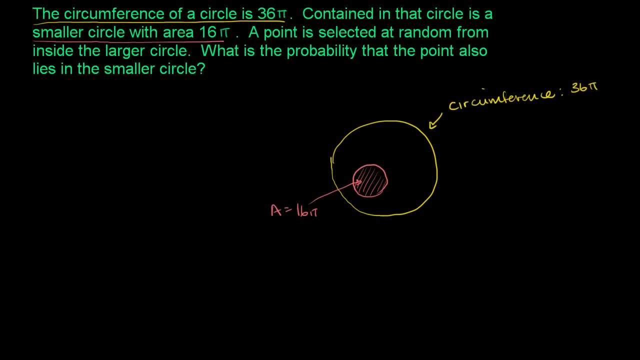 And we need to figure out the area of both of these circles. And so, for area, we need to know the radius, because area is pi? r squared. So we can figure out the radius from the circumference by saying: well, circumference, This is equal to 2 times pi times. 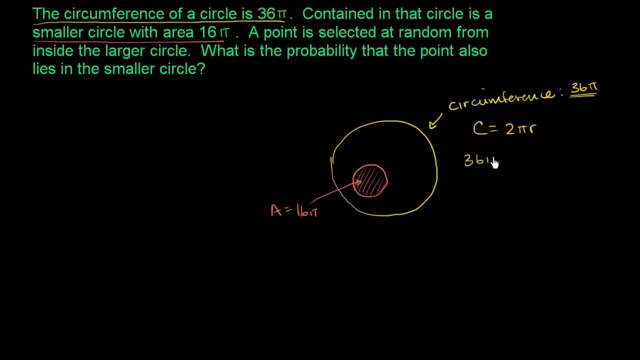 the radius of the circle, Or if you say 36 pi, which we're told is the circumference, is equal to 2 times pi times the radius. We can divide both sides by 2 pi, And on the left-hand side, 36 divided by 2 is 18.. 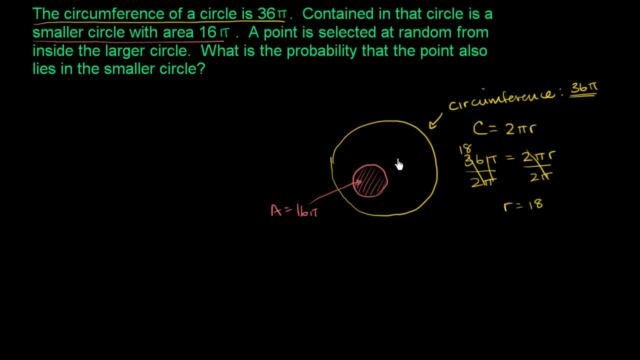 The pi's cancel out, We get our radius as being equal to 18 for this larger circle. This larger circle has a radius of 18.. So if we want to know what's its area, its area is going to be pi? r squared. 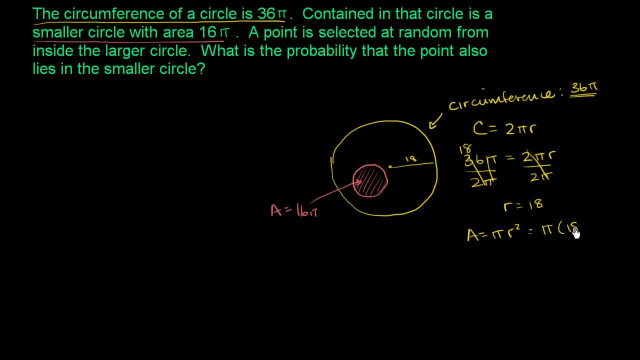 which is equal to pi times 18 squared. And let's figure out what 18 squared is: 18 times 18.. 8 times 8 is 64.. 8 times 1 is 8.. Plus 6 is 14.. 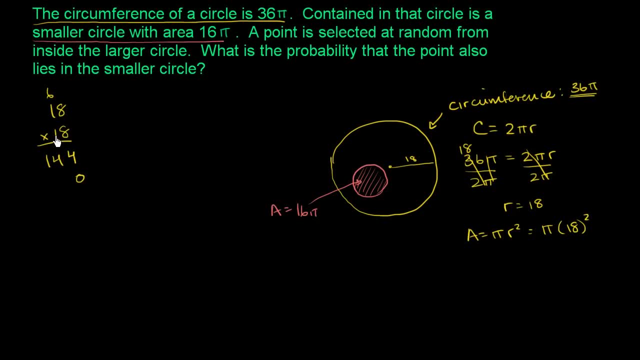 And then we put that 0 there, because we're now in the tens place. 1 times 8 is 8.. 1 times 1 is 1. And really this is a 10.. 10 times a 10.. 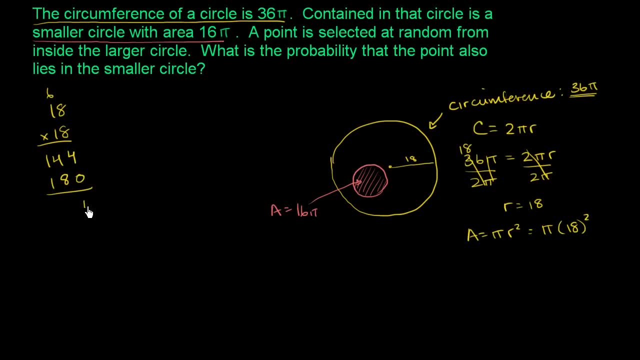 That's why it gives us 100.. But anyway, 4 plus 0 is a 4.. 4 plus 8 is a 12.. And then 1 plus 1 plus 1 is a 3.. So it's 324.. 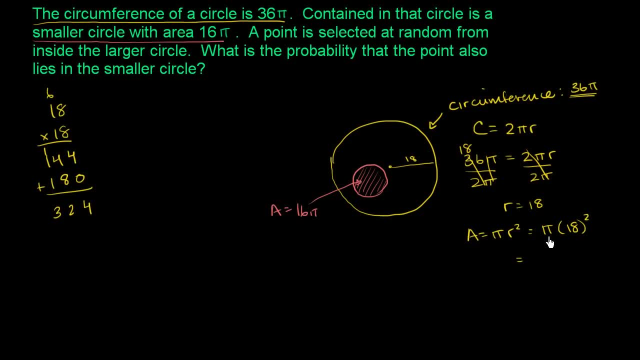 So the area here is equal to pi times 324.. Or we could say 324 pi. So the area of the entire larger circle, the part that I've shaded in yellow, including what's kind of under this orange circle, if you want to view it that way. 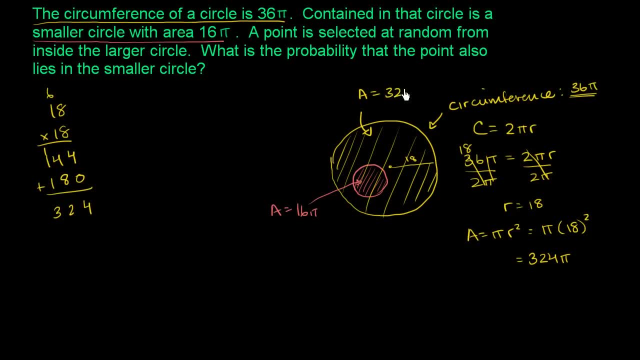 This area right over here is equal to 324 pi. So the probability that a point that we select from this larger circle is also in the smaller circle is really just a percentage of the larger circle that is the smaller circle. So our probability. I'll just write it like this: